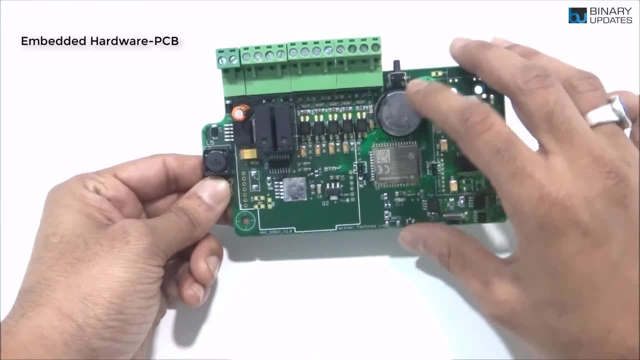 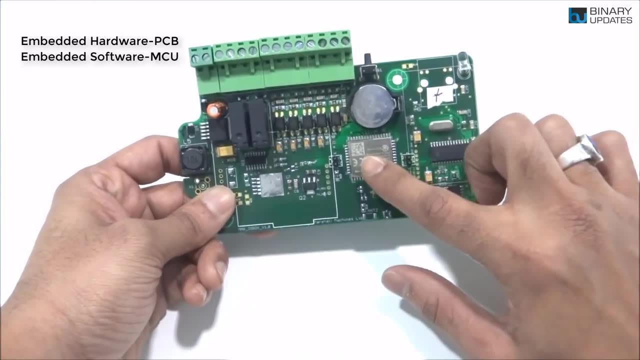 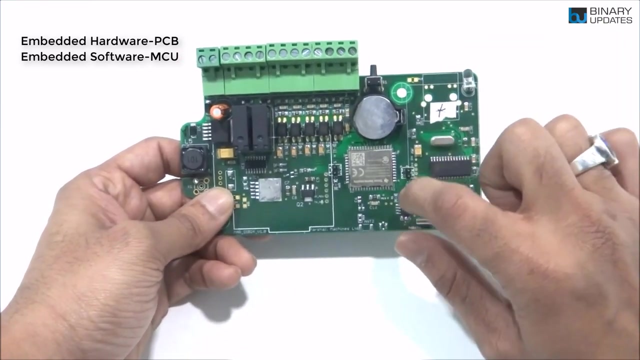 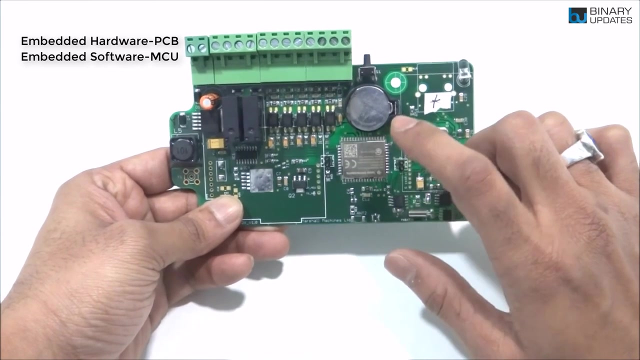 To layout and then place the components in order to function your electronic product properly. The second element to the embedded system is the microchips: a microcontroller, microprocessor and all of the programmable devices like FPGAs or something which you can write a program that's basically called embedded software. So this chips, the microcontroller and microprocessor chips- runs the piece of software that's called embedded software, which basically makes this. 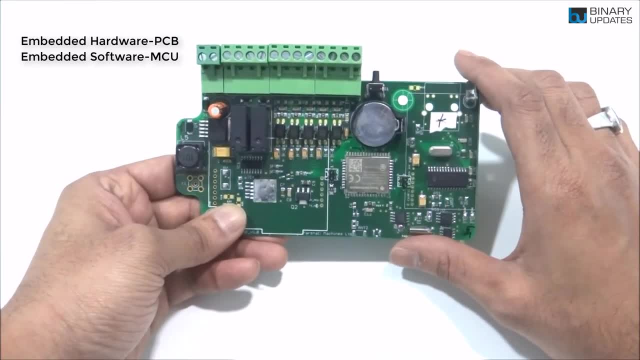 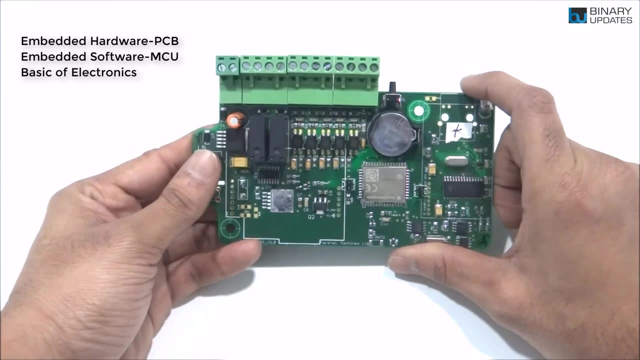 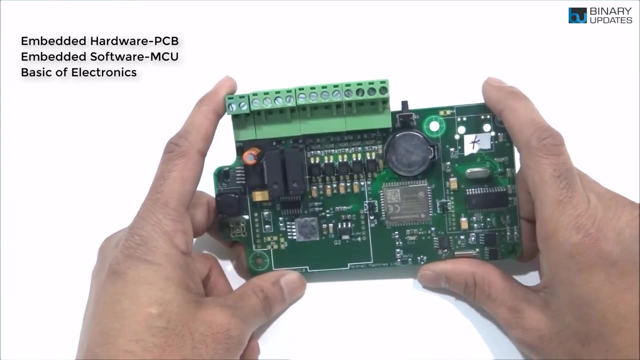 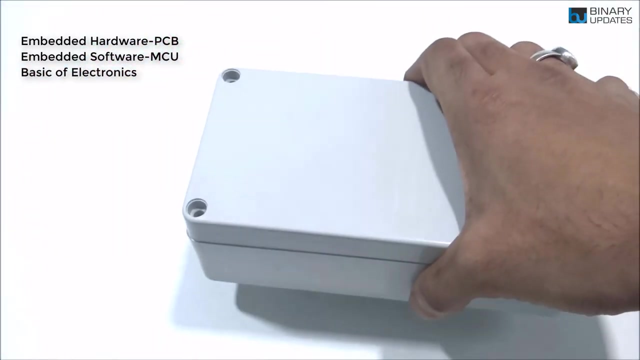 circuit board to work in order to control or monitor the data or something like this. Okay, and the third essential part is basically in the active and passive electronics components. So the one must have to know the basic electronics. Now, when we're talking about a specific product, then I can show you when this circuit goes into the production or when it goes to the client. it could be shipped with this kind of you know box. It's basically. 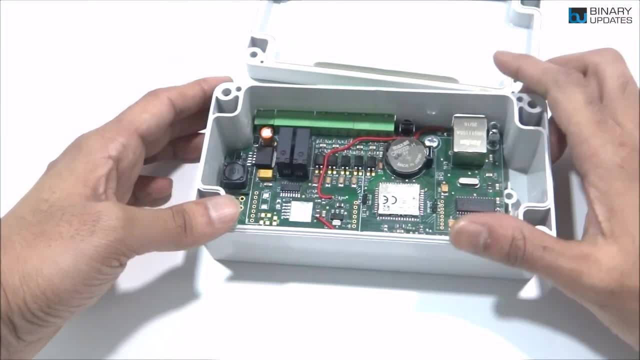 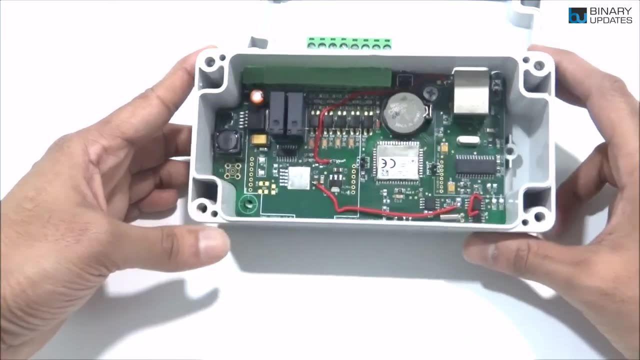 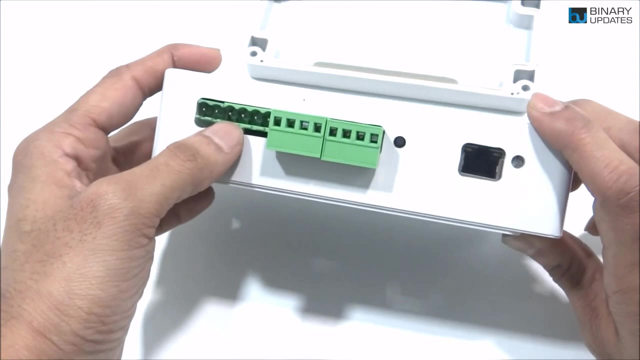 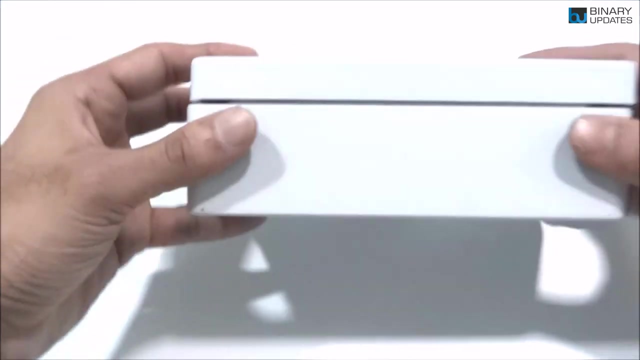 The parts in which we can put the same circuit board that I've designed and there is a little you know, cable you can see for testing and all in-house. We made it before we ship it to our customers and there's a connector- this where you can connect your easy components that you want to to connect and to monitor and control. So my point here is: this is how you know the products are made, This is how any embedded system products are made, and there's an Ethernet connector. 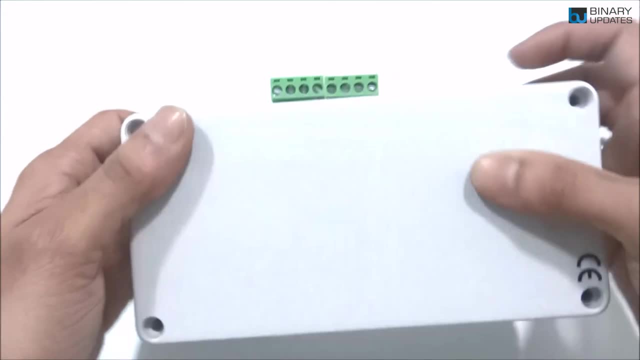 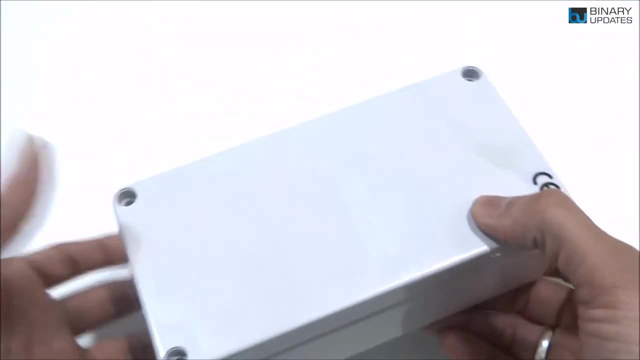 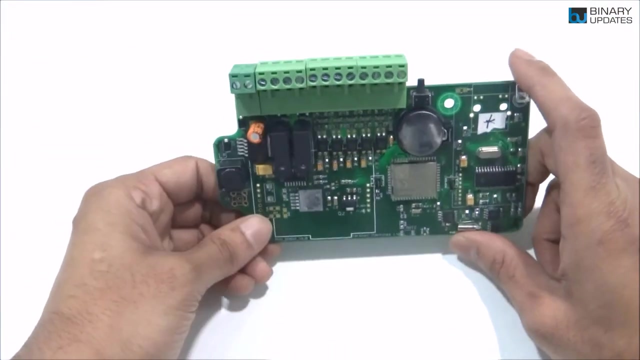 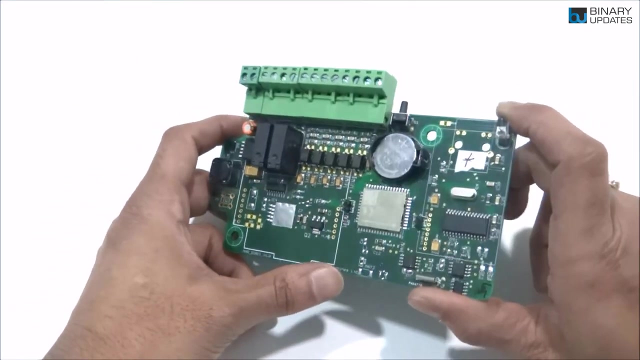 So LAN connector where you can connect your LAN cable and connect this device to internet. Basically, this is an internet connected embedded system product. Basically, you can call it as an IoT as well. So coming back to our previous discussions, So if you want to become an embedded system engineer and if you want to learn how to design this kind of product, then you must know there's three things: a PCB design.